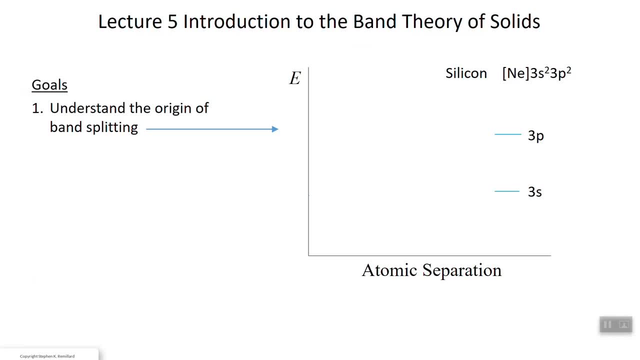 deeper and introduce the band theory of solids. To do that, I have some goals. First goal is really to understand the origin of why bands form, and so we're going to start just talking about silicon. If you look at the alfbaugh buildup of silicon, it's neon and two electrons in the 2s, 3s up shell. 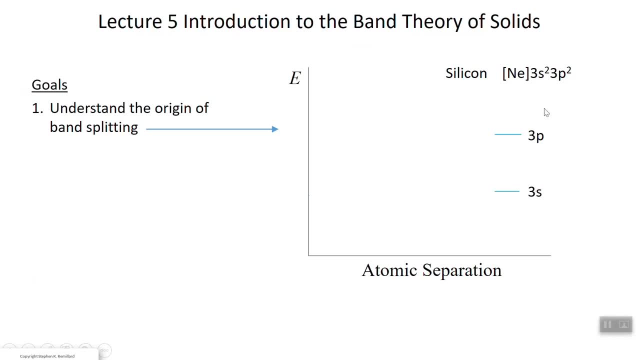 and two electrons in the three p sub shell. You know, those two subshells are not at the same energy. They're split by spin orbit coupling into two different energy levels, and so you might sketch just their energy levels like this: The three electrons that are: 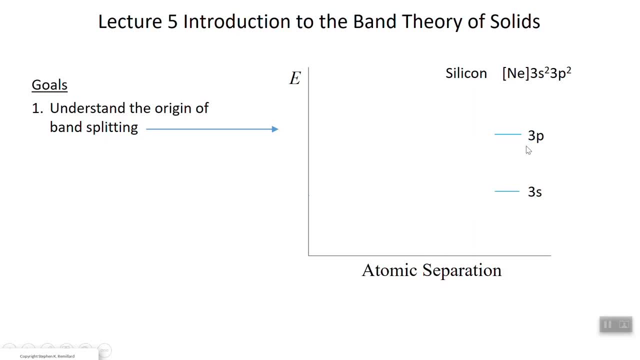 and the 3s subshell are there and 3p are there, and that's for a silicon atom, One silicon atom, all by its lonesome. Now, if I take two silicon atoms and move them close to each other, something interesting happens. So these are the energy levels as a function of how far apart these two. 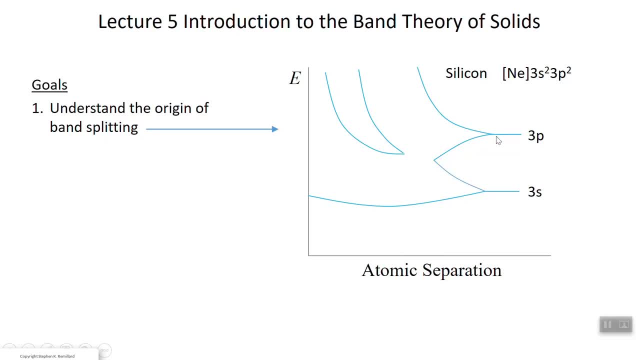 atoms are from each other. As the atoms get closer and closer they reach a point where you start to notice those energy levels split. So 3p splits into two levels. the 3s splits into two levels. I can't say which one of these levels is the left atom and which one is the right atom. It's both. 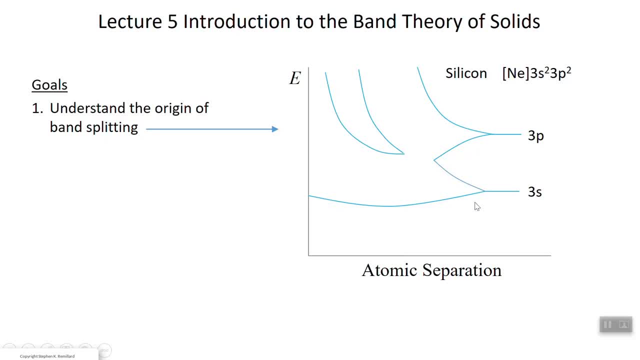 atoms. These are the 3p states and these are the 3s states for the system of two atoms. As I bring those atoms closer and closer together, I'll get to a point where 3p and 3s actually run into each. 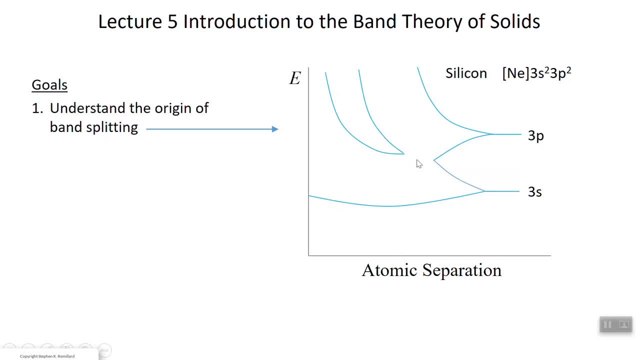 other and that, beyond the 3s and 3s, actually run into each other and that, beyond the 3s and 3s, below which there's no distinguishing them, and as I keep making them even closer and closer together, other other energy states are going to actually start to surface, and I'll get this. 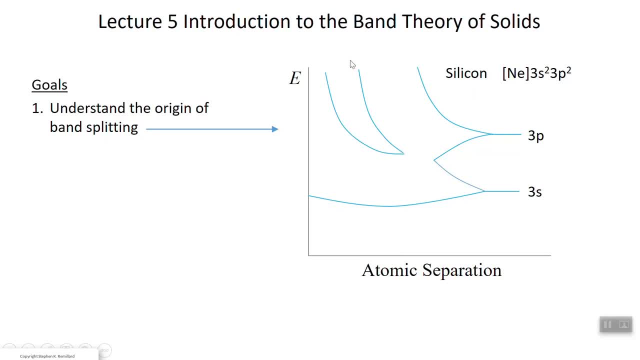 banana shaped thing where I just have these two, these two states possible. That's silicon, and we're going to understand why these splittings happen. Another thing that I want to accomplish right now is to understand just that conduction electrons are mobile and that valence electrons are not. It doesn't take a whole lot of 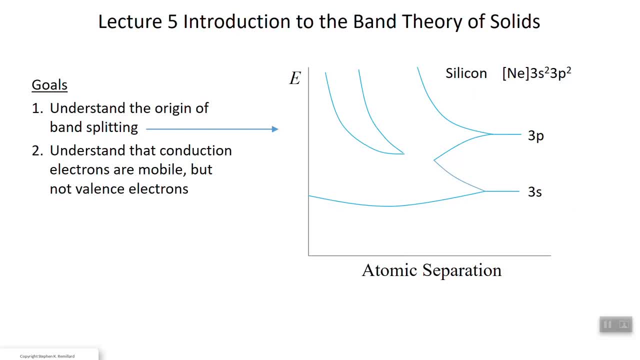 measurement. It's very heuristic Now. the valence electrons are stuck in the atoms, but we need to. we need to be really clear on that. What moves in a semiconductor are the conduction electrons and the holes. Holes can move and the movement of holes and the movement of conduction electrons are. 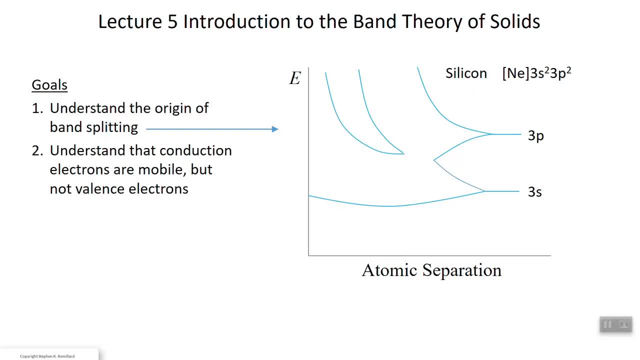 what give us the models we're going to develop for conduction through a semiconductor. A third goal for today is to interpret those energy band diagrams that you're going to see. This is not an energy band diagram, but we will get some And we want to be able to understand them All right. so those, those are the goals in hand. 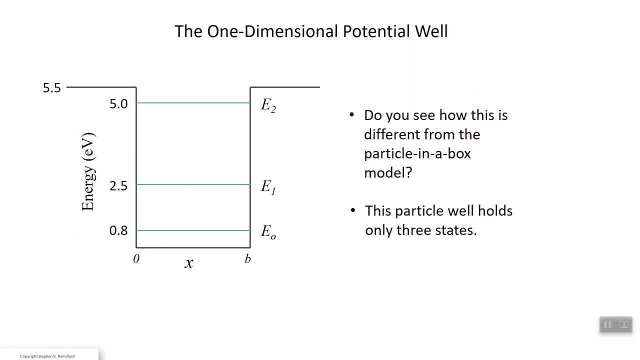 I want to start off by reviewing a problem from quantum mechanics called the one-dimensional potential. well, And it's similar to something that you may have seen- the particle in a box- and you may have seen this, the one-dimensional potential. well, They're very similar, except that. 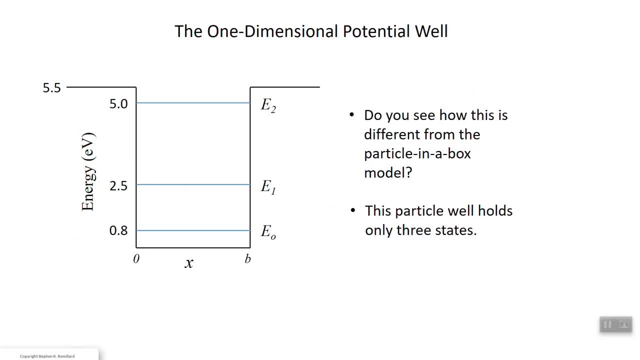 the one-dimensional potential well, is mathematically a messier, messier proposition. It actually comes out to have some very similar properties. You have a graph of potential energy versus position here. Potential energy of what? of an electron, for example? So an electron anywhere around here can have these potential energies between x equals zero. 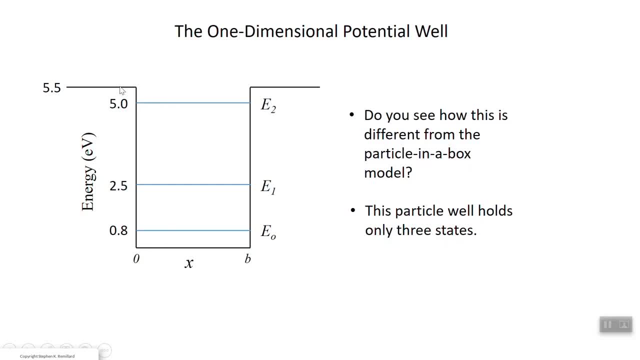 and b, It can actually have lower energies, And so you have a well, And if you have an electron with 2.5 electron volts of energy, you can actually toss it in this well and it will be stuck in it And it will stay right here at this level And there are only discrete energy levels that are 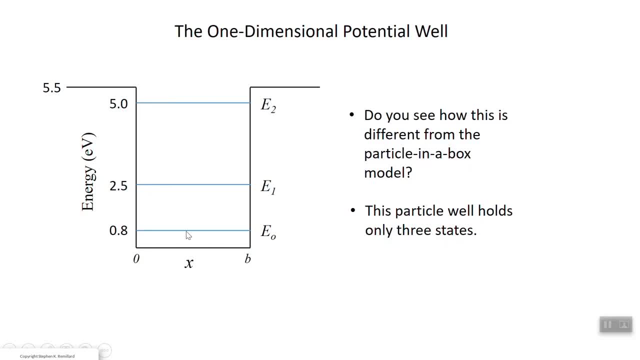 allowed. Just like you saw with the particle, This is a hypothetical well that happens to have a depth of five and a half electron volts, And so these three states fit inside, And you notice, as you get to higher levels they get farther apart. 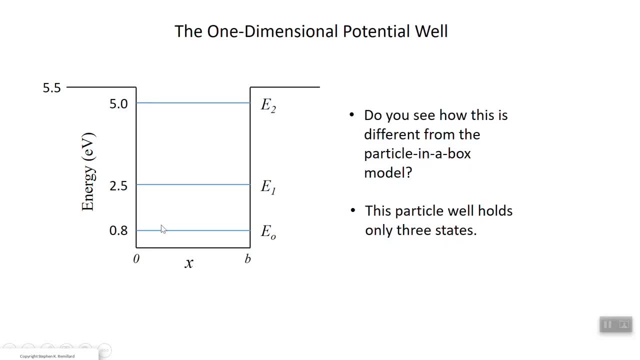 It's a lot like the Parthenon box, which I'll remind you about right here. A Parthenon box is basically an infinite well, is an infinite potential well, And so you have these energy levels that go as first the ground state and then the ground state, and then the ground state and then the ground. 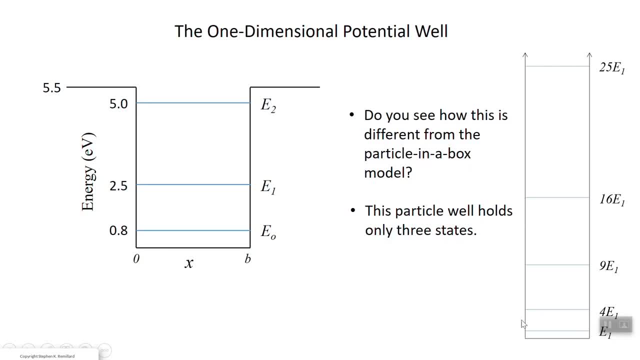 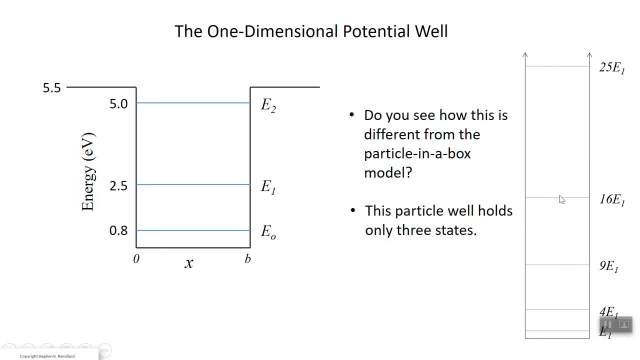 times the energy of the ground state. When n equals four, it goes as four squared, So on. So that's the, the Parthenon box, that is an infinite potential. well, So they're very similar. In fact, you notice that this almost is an n? squared, but it's a little different. You get a. 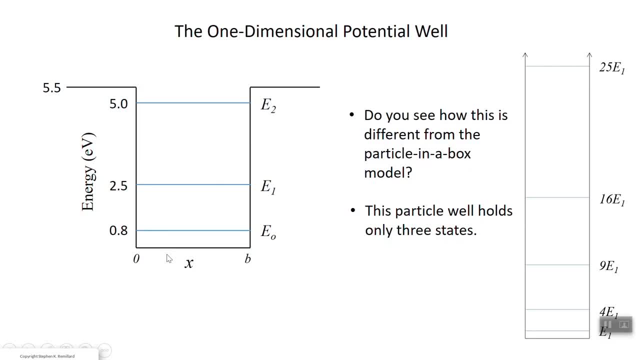 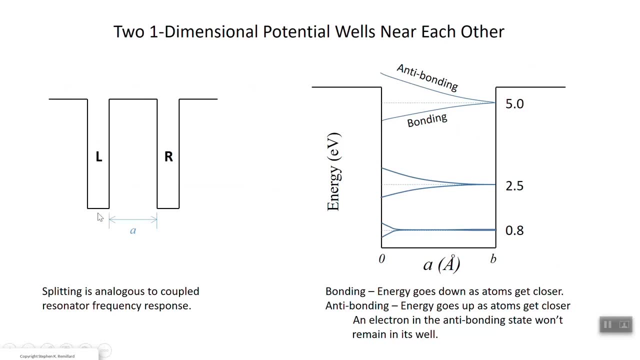 transcendental equation result there. I wanted to talk about this because I want to. I want to go into what happens when two quantum mechanical items get close to each other, So keeping with these potential wells, If I take these two finite potential wells and move them into close proximity. 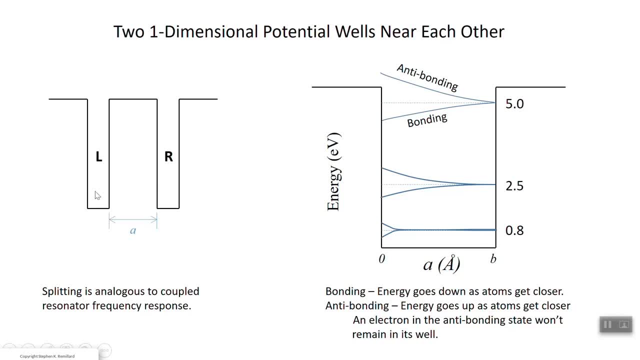 of each other, And so I'll call a the distance between the left well and the right well. Back to our well model, that is, potential energy versus position, and then the allowed states in between. Now these two palms, which arebn. they do this when they come into proximity, When 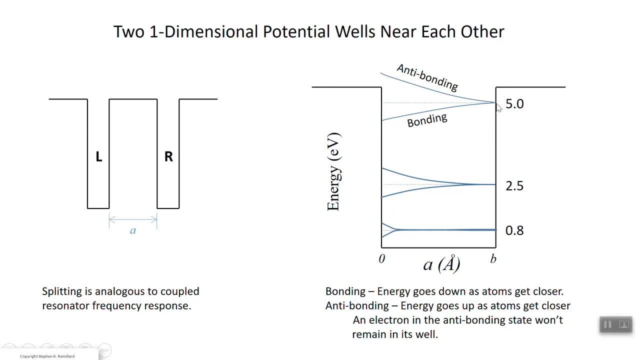 these two wells are far apart. you just have those 0.8, 2.55 electron volt energy levels. But when those wells get closer together, those energy levels start to split and you get one level that goes up and one level that goes down. It's not that one of these belongs to the left. 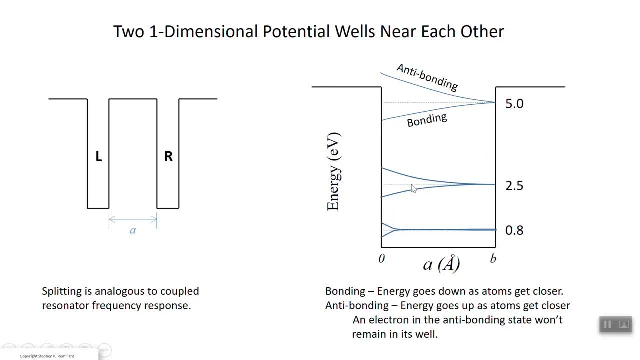 well and one belongs to the right well, These two energy levels belong to the system of two wells, And it becomes a more pronounced effect for the higher energy states, and so we'll just look at them to really make a sense of what this is all about. If I have 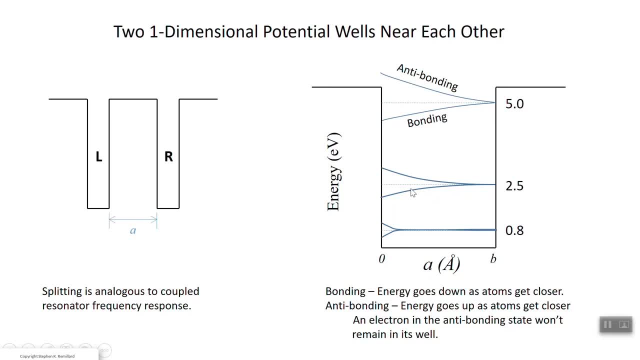 two wells in proximity. there are two different characteristics of these split-off states. One of them you call bonding and one you can call anti-bonding, and the reason why has to do entirely with energy. The energy minimum principle of physics says that systems always prefer the 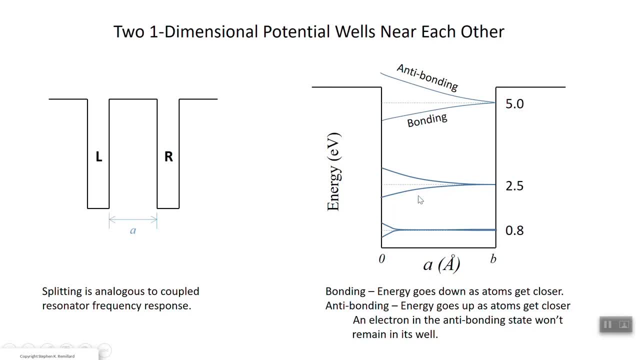 lowest possible energy. They always strive to minimize energy, right. So if I bring two wells in close proximity with each other, if they follow this lower split-off, then as the wells get closer and closer, the energy gets lower. That's favorable. Those two wells are going to be attracted to each. 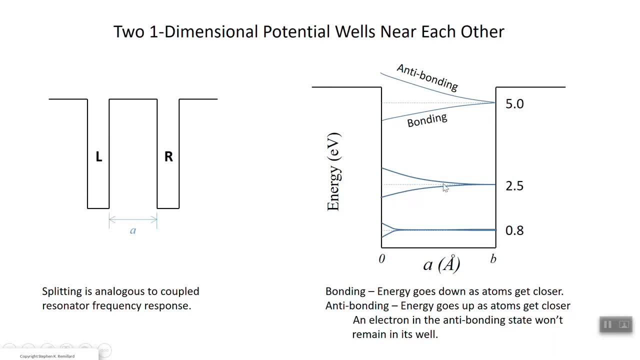 other. but if I bring two wells into close proximity and they follow this upper split-off, then as they get closer and closer together, the energy goes up. That's energetically unfavorable and those two wells will repel each other and that's why it's called anti-bonding as opposed to 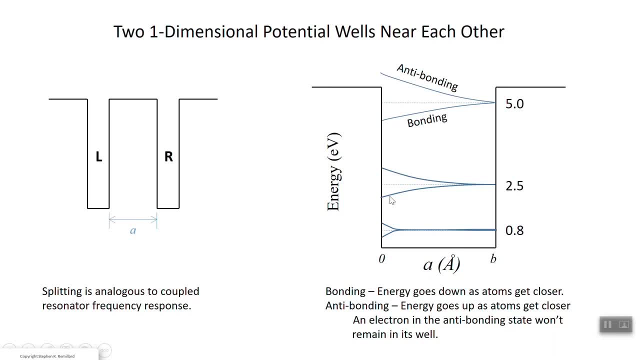 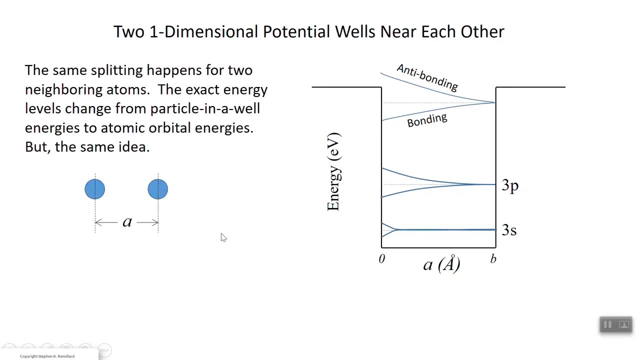 bonding Where they attract, And that sounds like a chemical thing, because the same principle is used to explain chemical bonding. If, instead of the left well and the right well, I put two atoms near each other, So here we have two atoms, with some separation When they're far apart, you know. 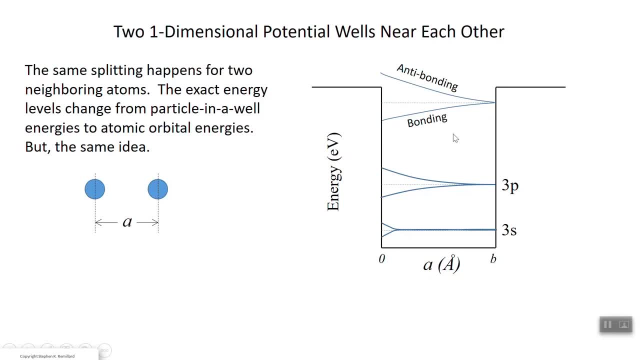 you have your discrete subshells And yes, let's talk about silicon, where you'd have these shells. You know that are filled. the 3s and 3p are two filled, outermost filled subshells. As you bring these two, 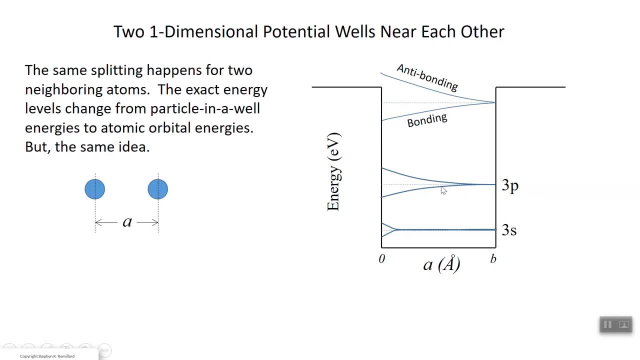 silicon atoms closer together, you start to see a split-off between the 3p subshell. The p subshell can hold six electrons In silicon. look at the alpha buildup. There are two electrons per silicon atom in the 3p subshell, meaning that when two silicon atoms come close to each other, there are 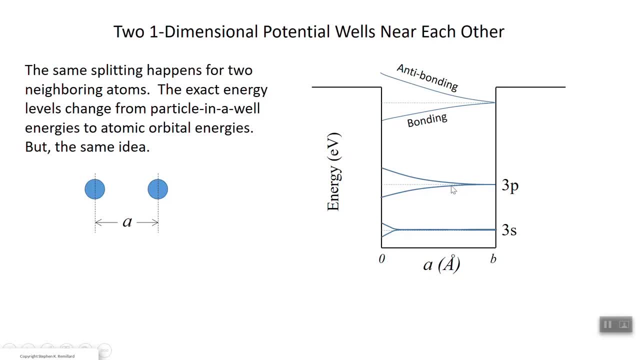 four 3p electrons And there's so meaning there's plenty of room for them in this lower energy level and they'll go there And you have bonding, And that's why silicon can form a solid. It can bond. You get these tetrahedral bonds. 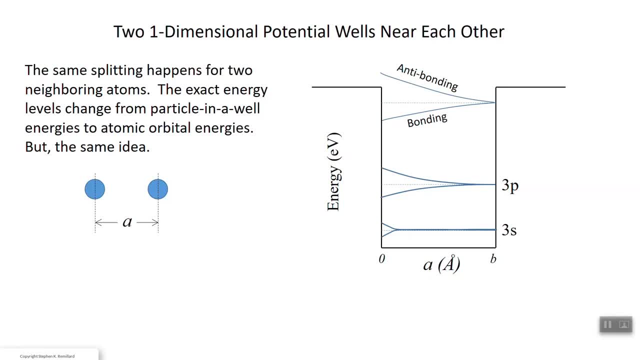 between silicon atoms due to the 3p electrons. As a counter argument, helium. Helium has a filled 1s subshell. So imagine this is a 1s subshell instead of a 3p. So helium's got two electrons in a helium atom and they fill up the 1s subshell. 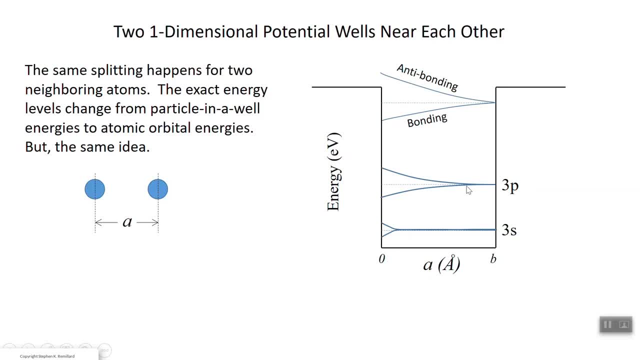 If you bring two helium atoms close to each other, there are four electrons. An s subshell can only, per the Pauli exclusion principle, hold two electrons. So, of those four electrons, two of them go into the lower one, but two of them go into the upper one, which, by the way, splits off more. So, two helium atoms close together, but two of them go into the upper one, which, by the way, splits off more. 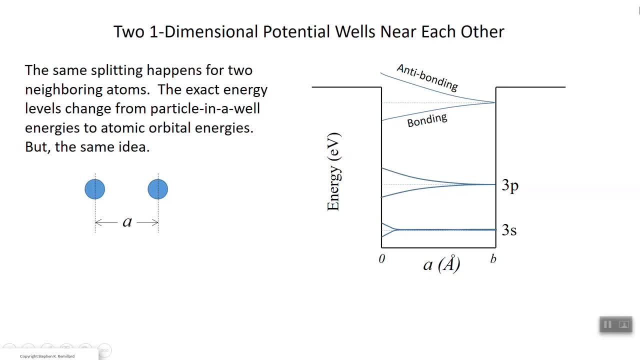 So two helium atoms close together are energetically unfavorable. Two atoms with filled the subshell are energetically unfavorable to be close to each other. So they don't form dimers. Helium doesn't. Silicon is just fine. Consider hydrogen. Hydrogen has one electron in the 1s subshell. 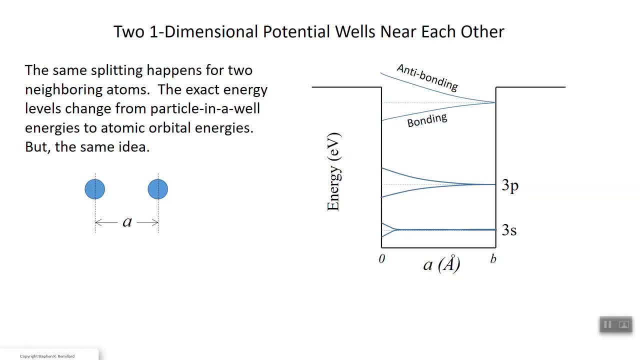 So you bring two hydrogens close to each other, you can get two electrons in this bonding split off per the Pauli principle. So hydrogen forms H2. just fine, Let's consider more than two atoms. So here I pictured five and I don't know if I got the right number of lines in there or not. but if you have five silicon atoms they will form additional splittings. 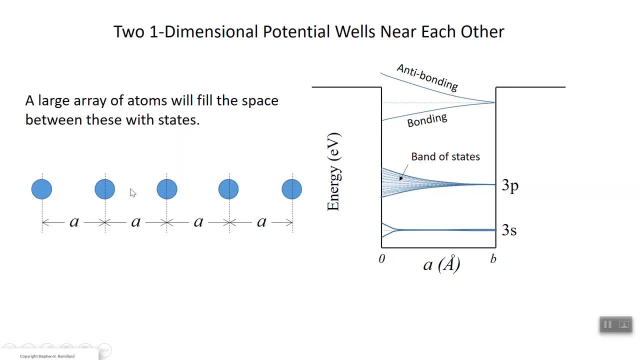 Because now not just adjacent atoms are coupled together, but non-adjacent atoms have a little bit of coupling, And so you end up with a lot of split-offs all between here. When they're just two, these are the split-offs, and when they're more than two, there are multiple split-offs in between those outer two that correspond to just two atoms. 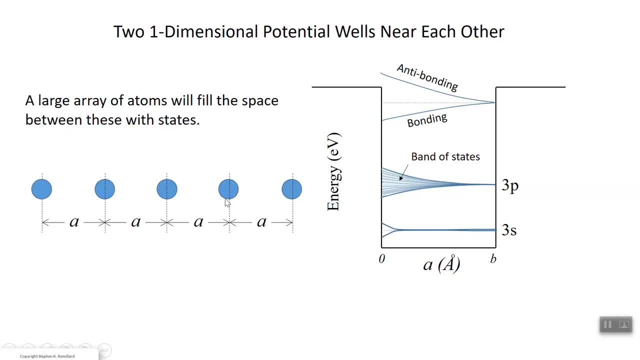 And this is an interesting thing, That's five. Suppose you had a solid, a bulk solid. so you have, you know, a 10 to the 20-some atoms, say 10 to the 21 atoms. If I had 10 to the 21 atoms, I'd have 10 to the 21 lines in here. 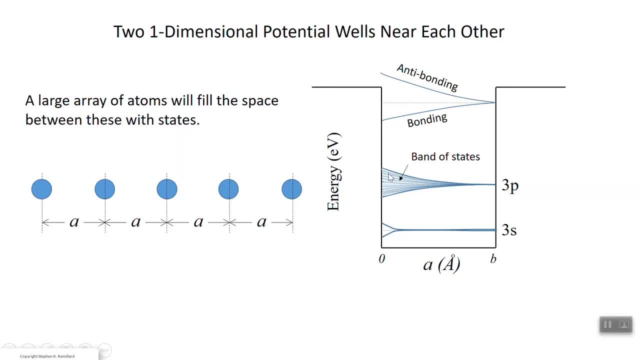 That's a lot of lines in that space. This will essentially be, then, a continuum In an actual macroscopic material. this is a continuum of states in this split-off, That's a band. That is a continuum of states, all of which can be occupied, none of which are assigned to a specific atom. 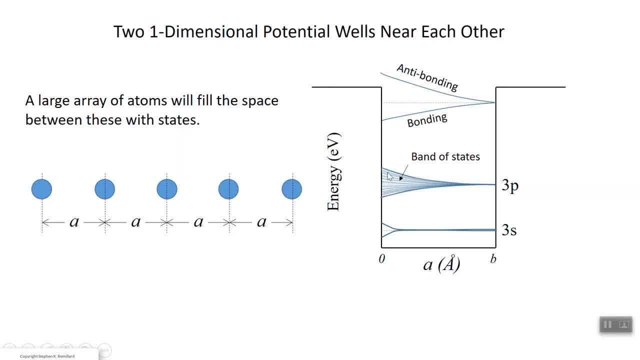 There are states of the system but each state can hold. well, if it's a P subshell for silicon, then it can hold six electrons. So you know there are, but there are a lot of states, so that's the band of silicon. 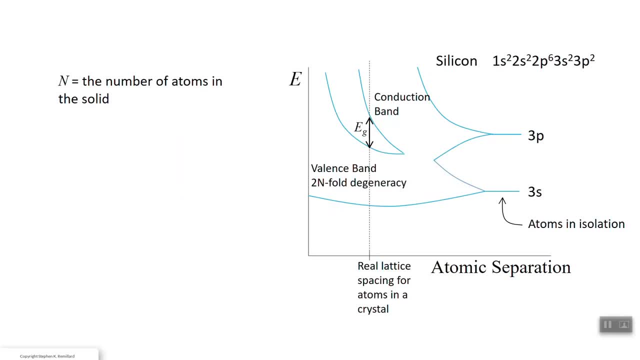 Let's go back to the picture we started with where for silicon, where we brought two silicon atoms closer and closer together and then they split off: the 2s splits into bonding and anti-bonding, and a 3p splits into bonding and anti-bonding. 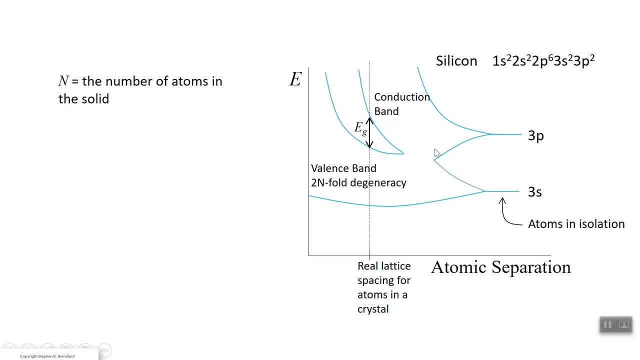 Eventually they get so close the 3p and the 3s merge together, but then at some point we get these additional bands forming. Now the thing about the banana-shaped pair of lines is The fact they have together is to take the energy levels that would be here and push them out of the way. 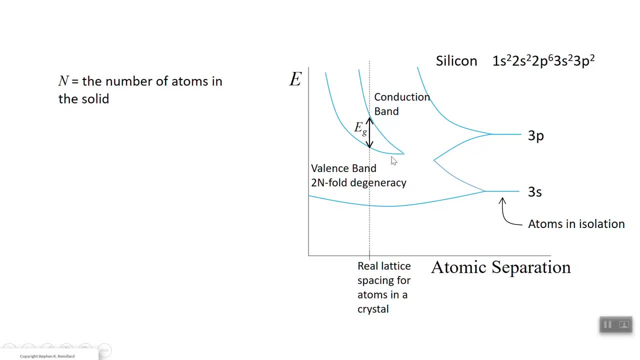 This thing is like a tusk that's been driven into the, into the kiln, and so there are no allowed energies inside of here, And so you have this bandgap, and that's what that is. That is a bandgap. 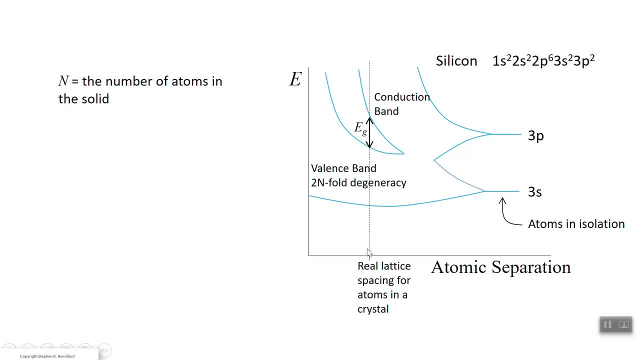 This is the real lattice spacing for atoms in the silicon crystal and their energy is down here. that belongs to an electricế ideas. That is right here. but if the PP gemeinsam is out and so on, and when OH is controlled, iano is out and when OH is, other angle of attraction is not formed, then we would know what ns plus would become. We also see the energy increase. as long as the energy is compacted, Yeah, that will not come to random스�, chemistry etc. 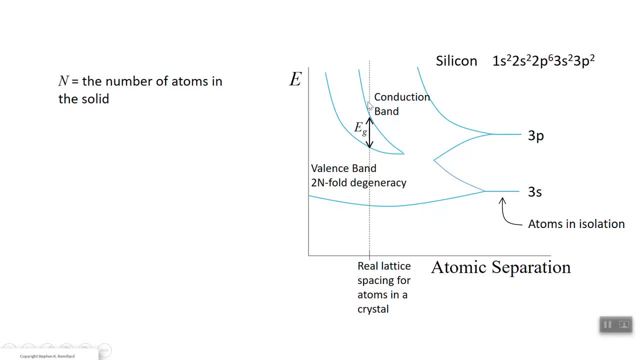 belongs to an electron that's bound in the atoms. If the energy is up here, that belongs to an electron that is free to move, And if the energy is in here, it's forbidden. And that's your band gap. Let's say there are n atoms in our particular sample of silicon. We'd say that the valence band 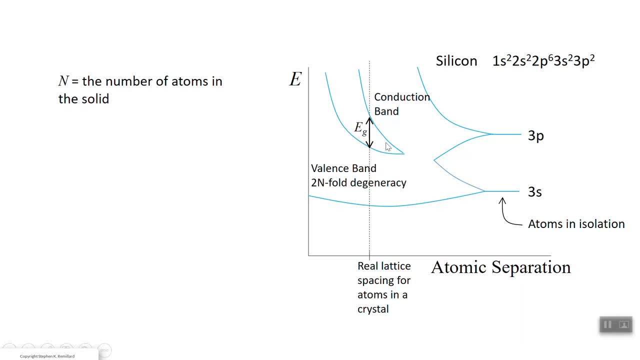 has two n-fold degeneracy because, per the Pauli principle, you have two electrons in each state And this band degeneracy- not maybe the state degeneracy you've heard about, which is multiple states that have the same energy, In this case, a band degeneracy is a bunch of states that 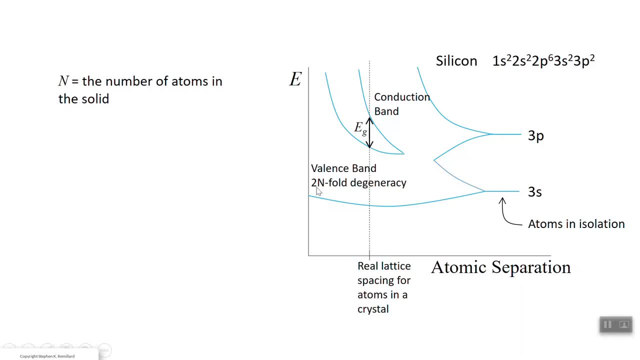 fit into a band of energies And there is two. n-fold degenerate And the conduction band will have far fewer electrons available but lots of states. If you have used the word degeneracy in a physics course before, this might be a slight. 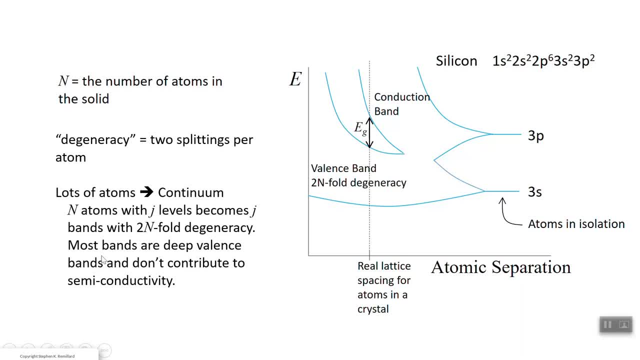 a different take on that term. We'll leave this little section down here for you to look at. It's what I just said, I think. Except, most bands are deep valence bands and don't contribute to semi-conductivity. So all of these energies down here are what you call deep valence And there 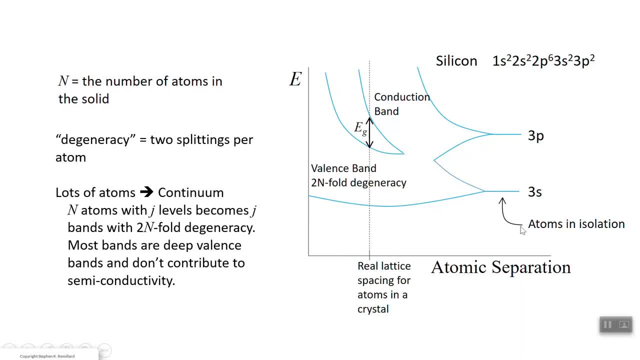 are actually more bands down here, right, Because this is a 3S splitting off And we haven't talked about the 2S and the 2P, But they're down here And so you are forming more bands down here, but they are all valence. 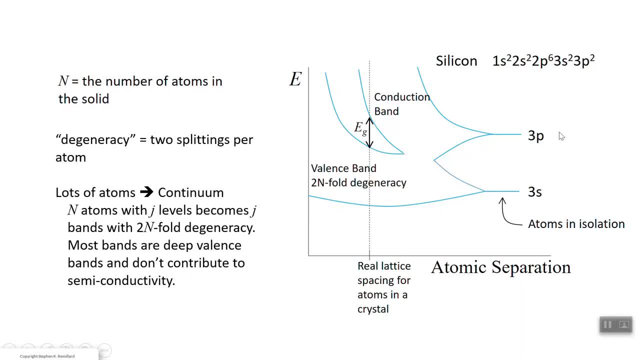 It's only way up here at the top of the half-pile that you have conduction. Okay, when we come back, we're going to look at real band diagrams, Because what you see here is not a band diagram. A band diagram is a little different. It puts this in what you call k-space. 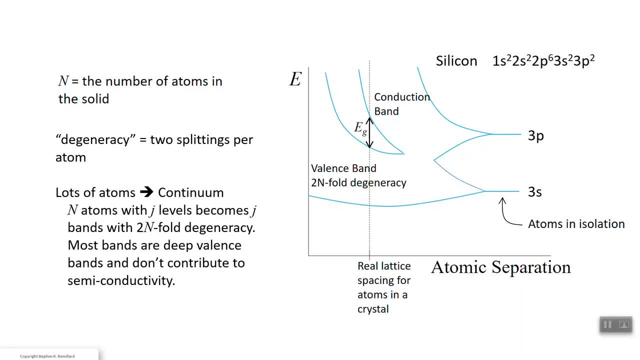 And we'll look at zero and one-dimensional band diagrams, which are much more intuitive, And we'll do that next time.